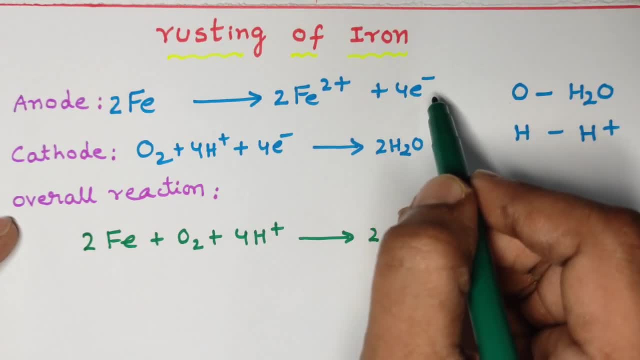 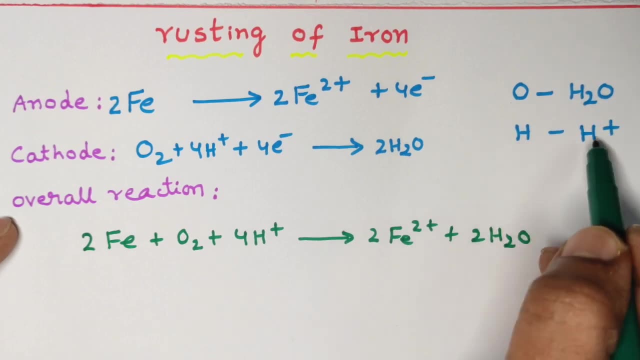 So two iron atoms are involved, so it losing four electrons At cathode O2, then how do you do it? Just balance the oxygen with water molecule and hydrogen with H plus ion. So two oxygens are there right side, two water molecules, Two into two. four electrons are. 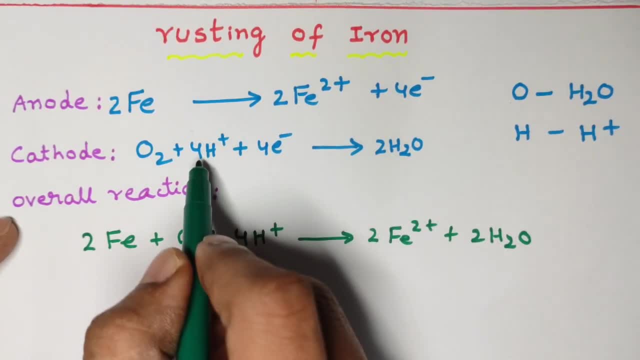 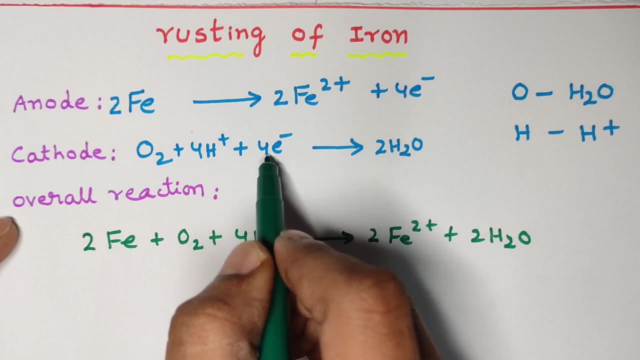 there Four, sorry four hydrogens are there. That's why left side four H plus ions you can write At anode it losing four electrons. right At cathode it is gaining those four electrons. Overall reaction. just you can combine reaction at anode and reaction at cathode. I hope you. 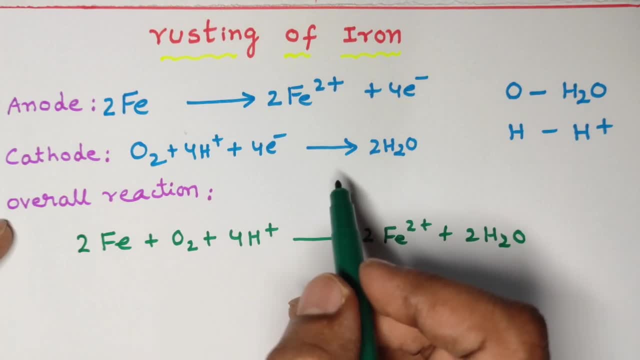 understood this. Please subscribe our channel and share this video to your friends and classmates. Thanks for watching. Love you all, Bye, bye. 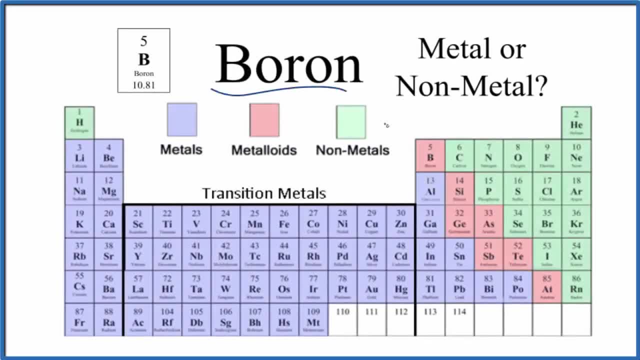 In this video we'll look at whether boron is a metal, non-metal or metalloid. So we have the periodic table here and the trend is that on the left we have metals. So most of these here on the left side they're metals, with the exception of hydrogen That is a non-metal. You have to watch out for that. 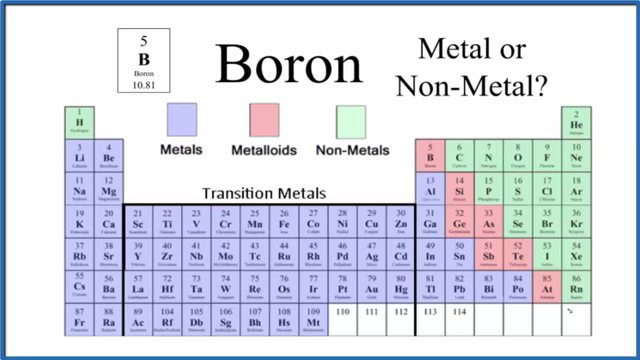 And then on the right we have our non-metals And in between we have what are called the metalloids. They have properties of both the metals and the non-metals. Boron, right here, it is a metalloid. 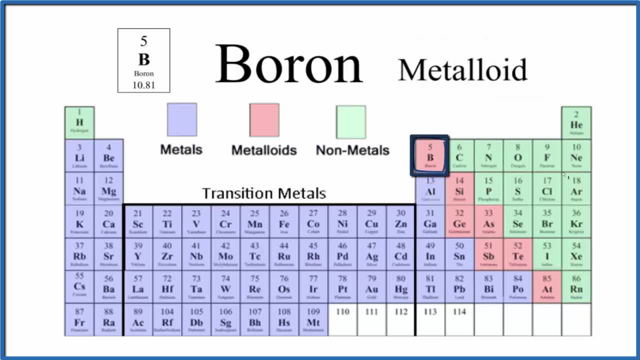 So it has properties in between the metals and the non-metals. Probably the easiest way to remember is we have on the left here the metals, with the exception of hydrogen, on the right the non-metals and in between we have the metalloids like boron. 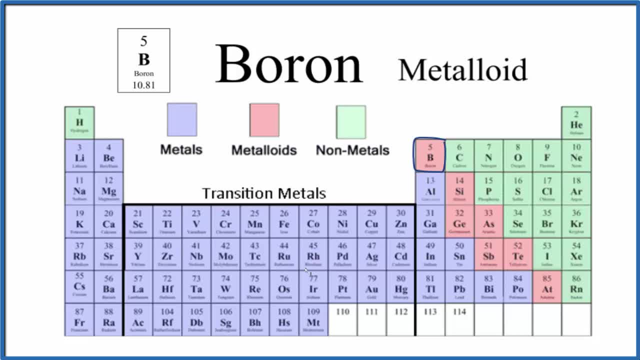 You really just have to memorize the metalloids and then you'll know. the metals are on the left, non-metals are on the right. But in answer to our question, boron is considered a metalloid. This is Dr B. Thanks for watching.